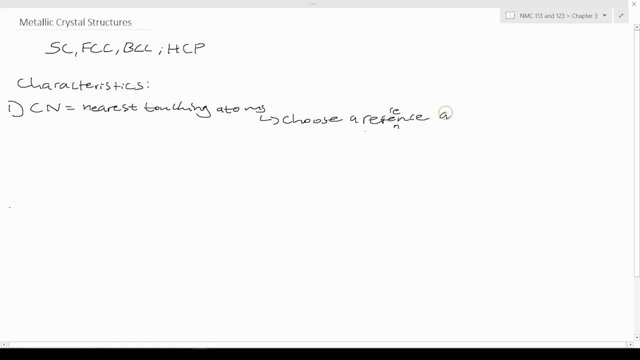 Vehicle력ing element, Vehicle française atem. You choose a reference atom within the unit cell. Secondly, what you do is you count the atoms within the shortest distance from the reference patient. You figure out the ELIP, donc you look up theigo to the centre of the reference atem. 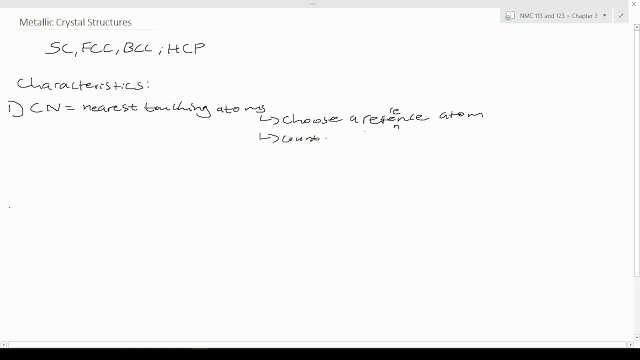 Secondly, you launch an object. So basically you end the sequence on the number three. You do the Messier encont error, fake atem static. So basically you count the atoms within the shortest distance from the reference atem. You pick up the A to V, then look up this in E. 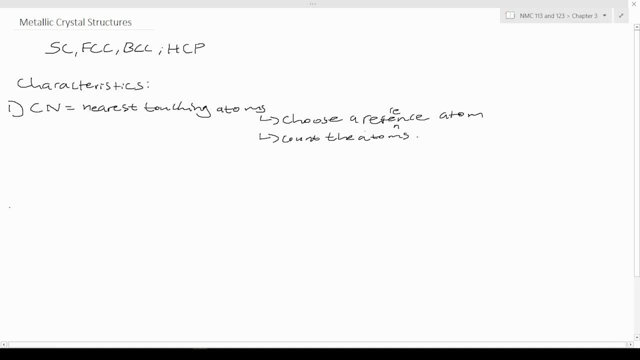 If we have enough left over. Hence, whatever number we have here, we may count the numbers in this system: Number runner: equal Number. Number Under confidence Number Raiserло: age four times Hub within the shortest distance from the reference item you've just chosen. 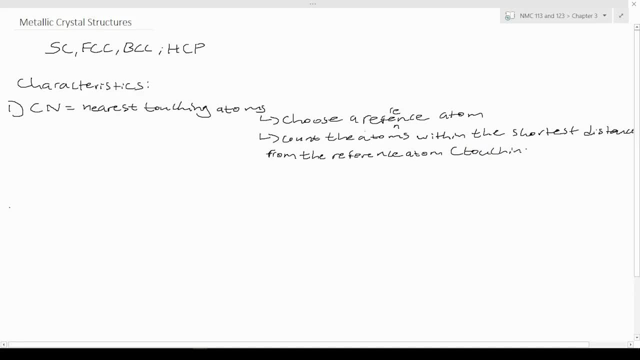 Secondly, another characteristic you need to be familiar with is being able to find the effective number of atoms. Effective number of atoms, Effective number of atoms within a unit cell, And this constitutes a total number of atoms within a single or within a unit cell. 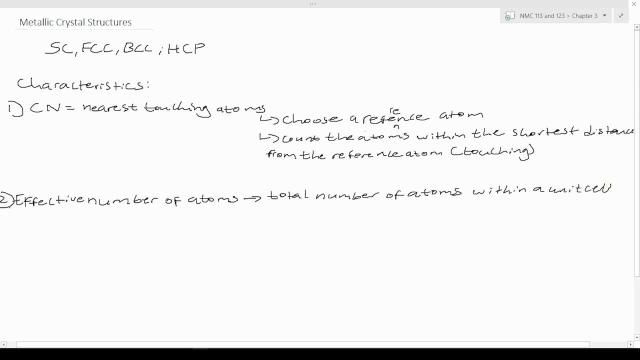 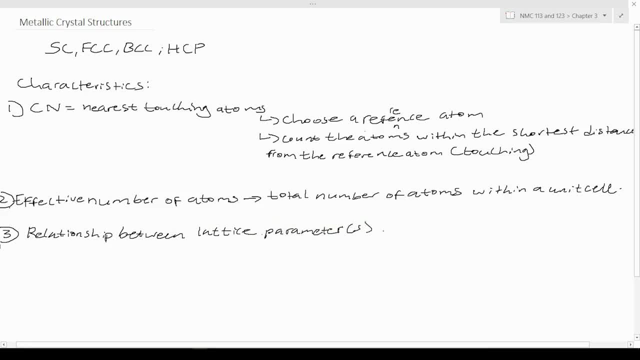 Uh, and the radius Atomic radius Radii, radius, Radii, radius, Radii, Radii, Radii, Radius, Radius, Radius, Radius, Radius, Radius, respecto, we're going to also, you only also going to have to be able to calculate the. 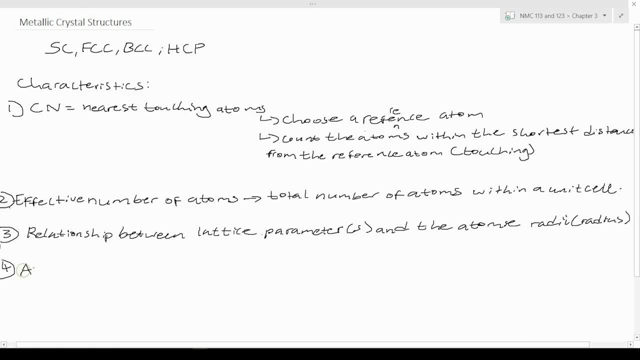 atomic packing factor. that's the atomic packing factor. it's normally abbreviated as a pf right and this is the total, the total atomic volume or the unit cell volume. this volume, that total atomic volume, what it means is that it's actually the effective, effective number of atoms right multiplied by a volume of a sphere. 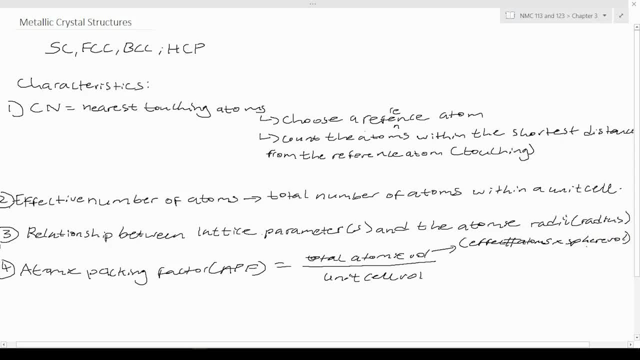 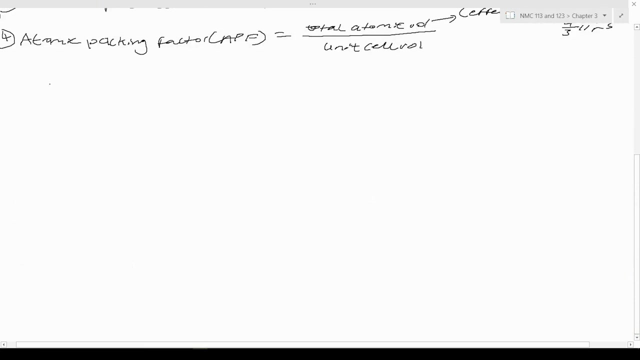 this is actually what the total atomic volume entails. so, as we know that the volume of a sphere is um four, three pi r cubed, okay, um, now we're going to look at the, the crystal structures individually, but first let's start with the simple cubic, simple cubic, uh, crystal structure. 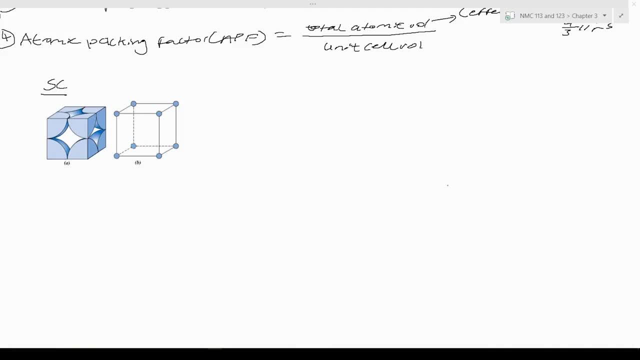 so here we have the, the unit cell for a simple cubic structure. um, now let's actually determine the coordination number, the coordination number for the symbol cubic. so now, in this unit cell, each, uh, the first thing i said you do is that you choose a reference atom. uh, you only have corner atoms, so you have to choose. 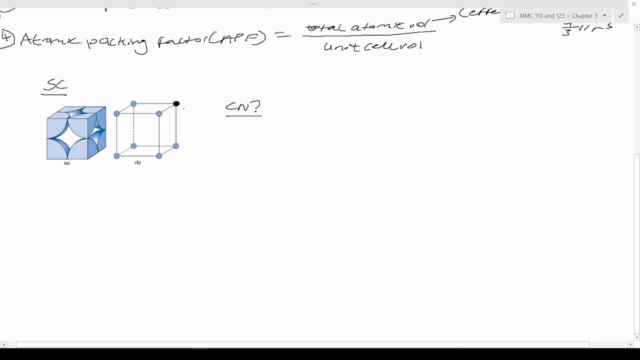 one of the corner atoms as your reference, as in, and then you look for the nearest touching, nearest touching uh atoms. so now, if you extend this unit cell, there are other surrounding unit cells because, remember, a crystal structure is a sequence right of a combination of a number of: 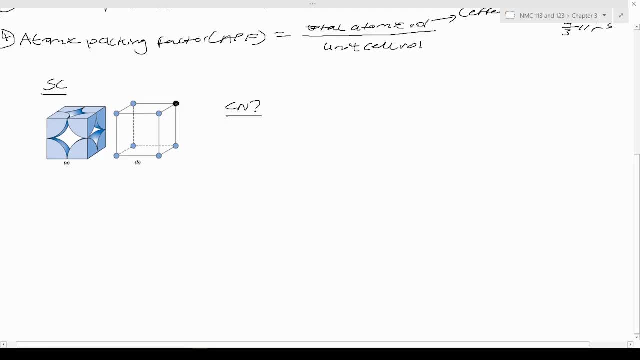 unit cells. so, um, with that in mind, you know that, actually, according to this, you have another unit cell, or a number of unit cells. so, um, with that in mind, you know that actually, according to this, you have another unit cell at the back right, and then i'm not gonna go draw there the entire unit cell. 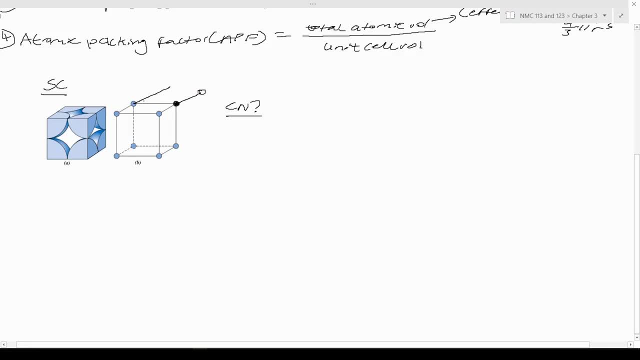 but, um, here you have an atom right, and then at the top- sorry, just excuse my drawing, it's a bit, you know, squeaky- um, you have another item here at the top, for the, for the, for the unit cell at the top right, and then on this side, on the side of this one, you also have another unit cell right, and 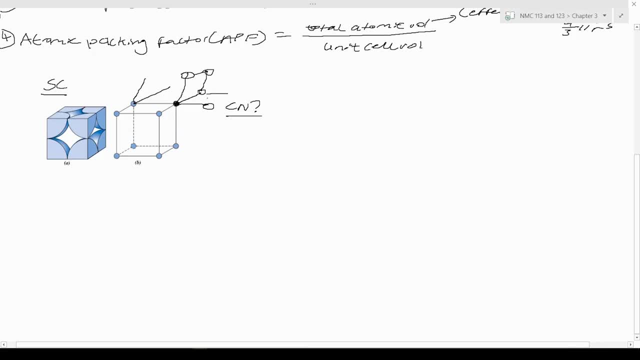 then this is the bottom unit cell that you have. you just extend this. right now the nearest touching atoms is actually um one. from here to the to that atom, to this one, that's two right, and then from here to this atom is three, and then the atom at the bottom here going down here, you have four, and then this is five. 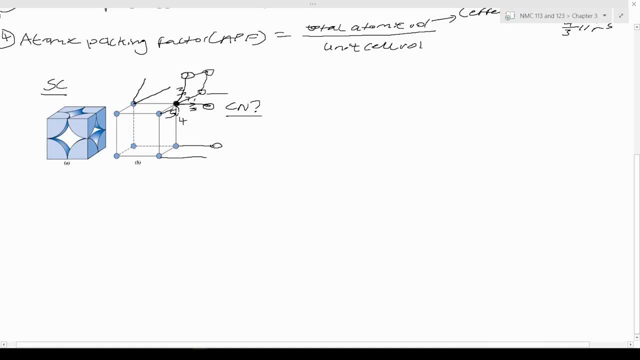 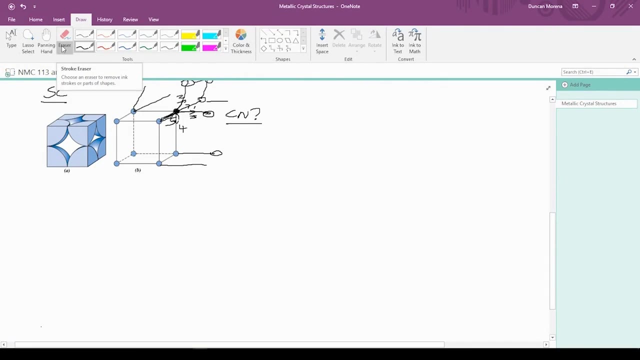 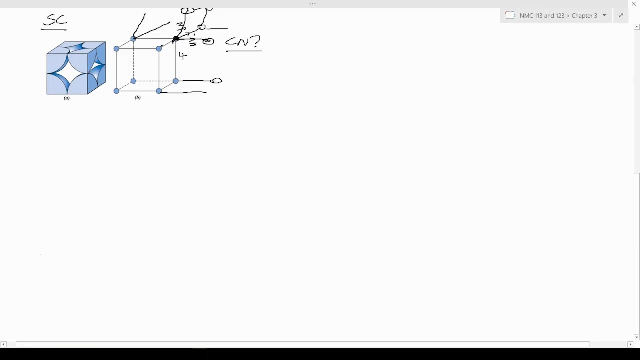 this is five. hopefully you can see, because, uh, my, my drawing pen is quite, this is the fifth one. let me just erase this. just find an eraser. okay, okay, yes, okay, now this is much better, okay, uh, okay, from here to here. right, we said it's, it's five, it's the fifth one. and then from here to 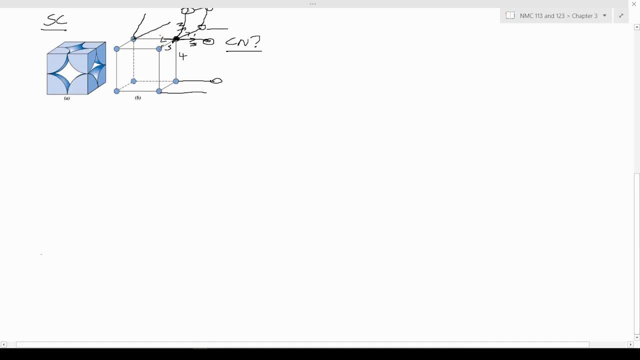 that side, that this atom, because it's also attaching that item, it's six. so you'll see that it's one, two, three, four. right on this, right on towards this atom, that's four, and then five and then six. so those are the the nearest touching atoms for this particular reference atom, which is a corner atom. 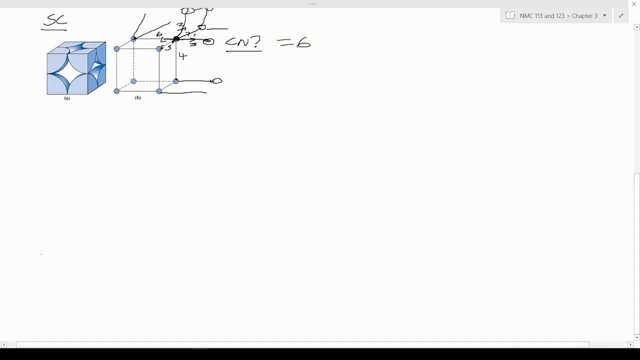 so we have a coordination number of six in a simple cubic and then, uh, the next thing we do is actually determining the effective number of atoms. now, we are now looking at thoughts, but you know we are not, then what we're going to do? now we are. 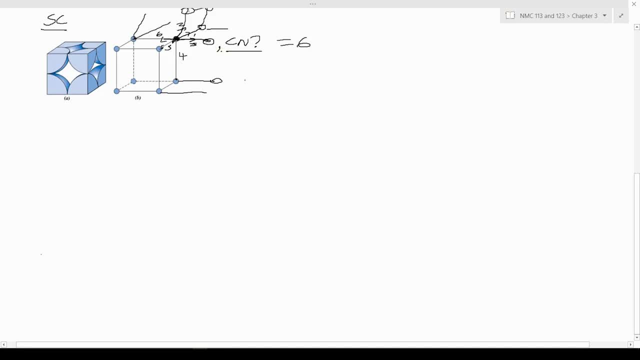 just going to keep going, so, so let me just do this. okay, this is the first thing that we did. now, okay, the second thing: uh, can get the effective, effective number right Now. the first thing you have to do is that you also look at what type of atoms you have. 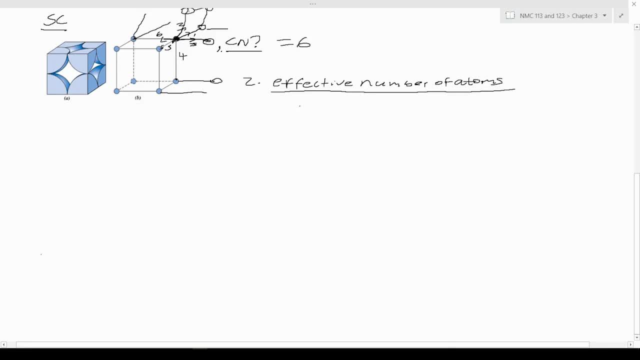 What I mean by that is if you have corner atoms, body centered atoms, like the orientation of the atom inside the cube. Now you only have corner atoms right, And then corner atoms have what we call a contribution factor. So you must actually determine the contribution factor of the corner atoms. 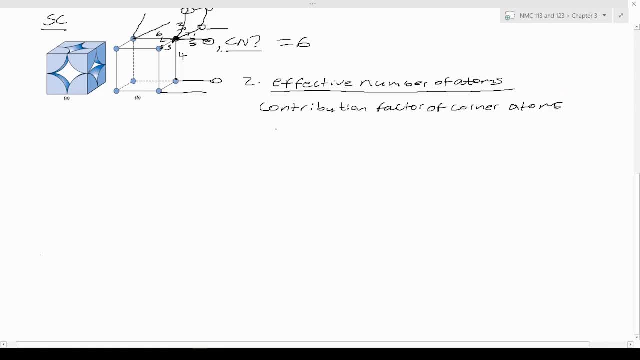 Those are the only atoms that you have. And then, after you determine the contribution factor, You have the contribution factor. So you have to actually get how many atoms are there right? So you have 8 corner atoms. So the number of corner atoms in this context, 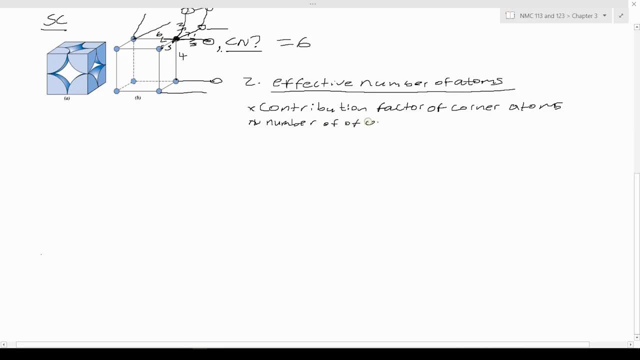 You get the number of corner atoms, Or effectively the number of atoms within this unit cell, But we only have the corner atoms. Hence I'm using that today To delineate to you how to determine the effective number of atoms. So the effective number of atoms. 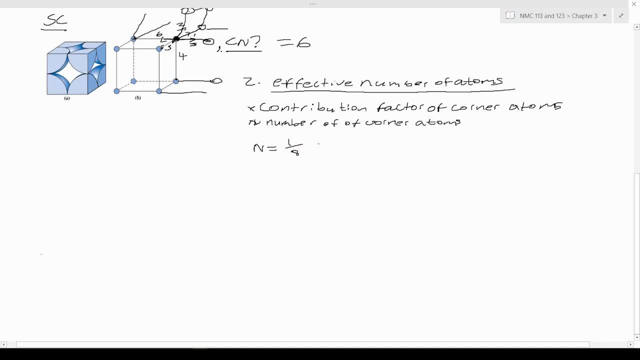 Which corner atom has a contribution factor of an eighth right. And then you have 8,, 8 corner atoms, And that means that the total number of atoms within this unit cell is one atom per unit cell. And then you have 8,, 8 corner atoms. 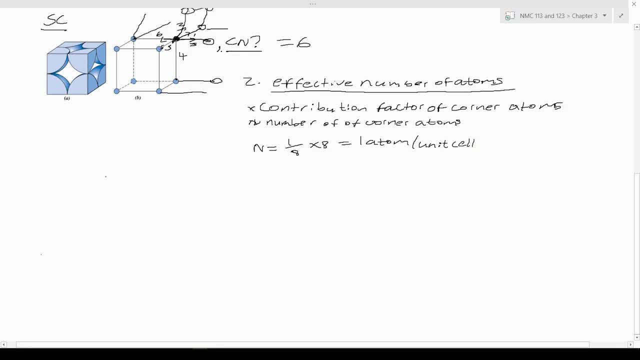 That's the real böl Spe virus dot bend. So this is what we earlier were going to do. The equation is that this: you get an accurate, full count, And that's that one parameter, And all of these things, And then Actuallly understand, Because whatever We do Really just going to look and sort these stuff. So just Aist U explicberries And then Um, Secondly, I mean thirdly- sorry, this looks a bit, uh, disorganized. 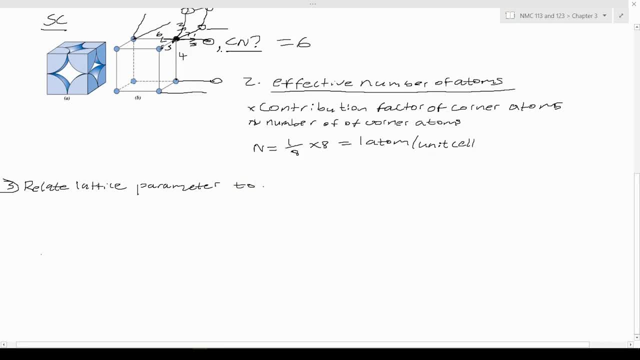 to the, the radius that's atomic, atomic radius right in this. in this case, if you look at the the sketch, when you this sketch on the left hand side of of the stick model, this is a stick model and then this a the sketch. here you can see. 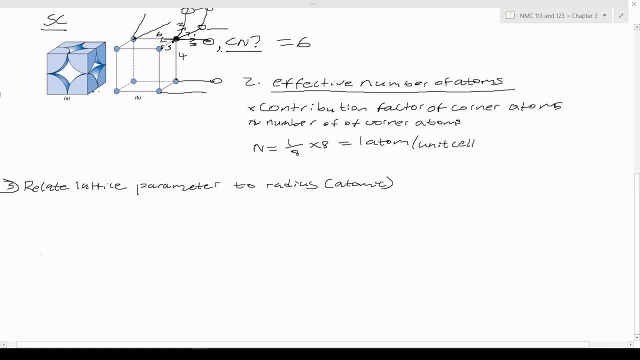 that these items are actually touching each other. and then this is the lattice parameter. this is a. from here to there it's a, it's just like here. this entire distance here is in fact a right. and then if you look at this particular drawing, that entire distance there it's actually a. now you can see that this is. 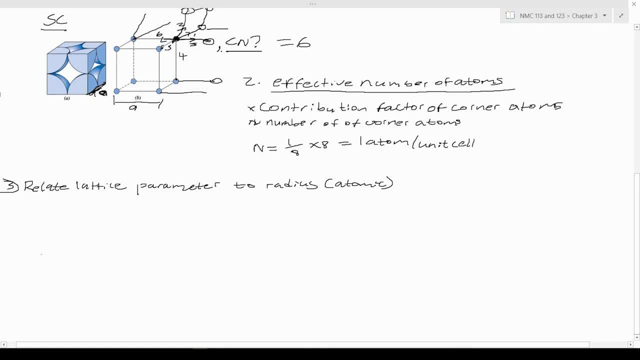 a full radius. from here to here is a full radius, and then from the next atom towards the edge, it's another radius. so you can actually say that, because of that, a, which is the lattice parameter, is equals to two radii. right, that's the relationship between the lattice. 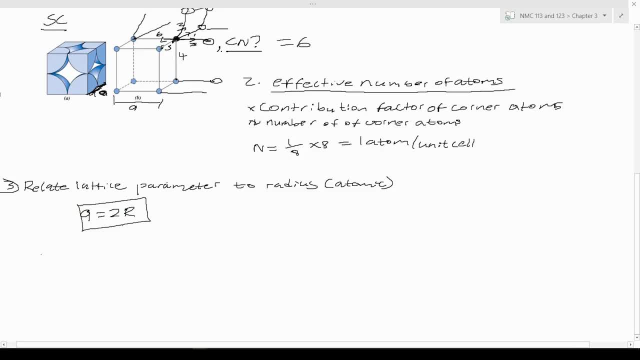 parameter of this cube to the radius. and then now, fourthly, you have to determine the atomic packing factor. we say that that atomic packing factor is total, total atomic atomic radius right within the unit cell and over, okay, our volume volume, right? no, no, sorry, I just made a mistake here. we just erase. 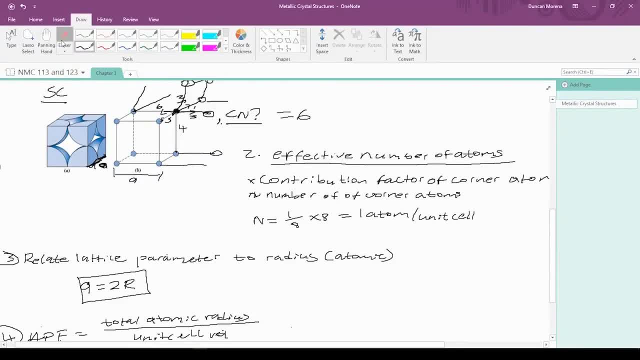 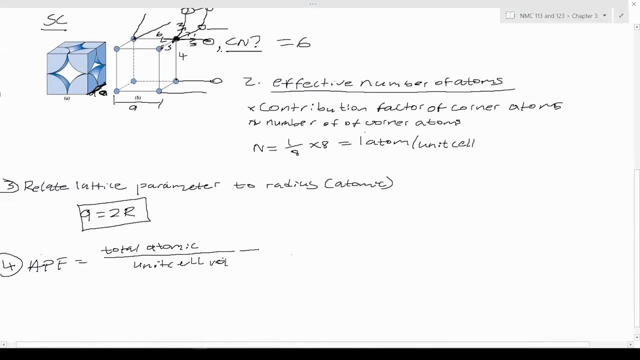 it. this is total atomic volume, not atomic radius, just excuse that. okay, let's blow this up: atomic volume, which is basically just the effective number of atoms, right, multiplied by, let me just say, effective number of atoms. I'll just abbreviate effective number of atoms multiplied by a sphere volume. 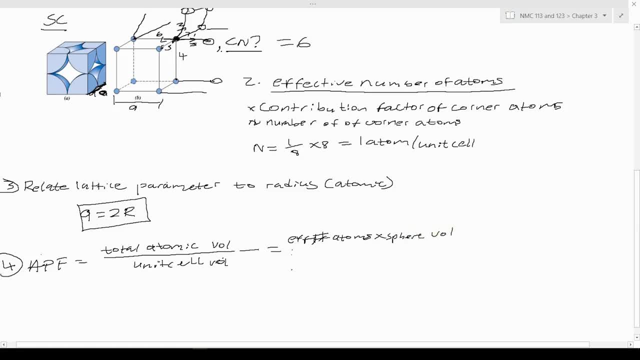 right, and this is all the unit cell volume. so we have the effective number of atoms, p groups. so it's one right. welcome to passengerish units. so oh, oh well, unit, yeah, unit cell multiplied by PI. forgot the four by three here. R cubed right over a cubed, because a the 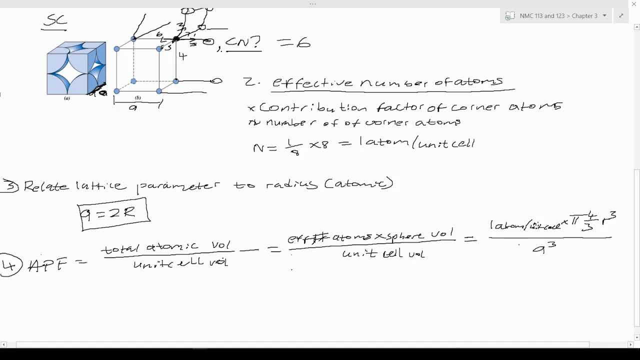 lattice parameters is a cube, so the volume of a cube. since the parameters are actually, they're just the same. that's actually why we just saying a cubed and you can write the radius for the bottom, the denominator in terms of the radius, using the relationship between the lattice parameter and the. 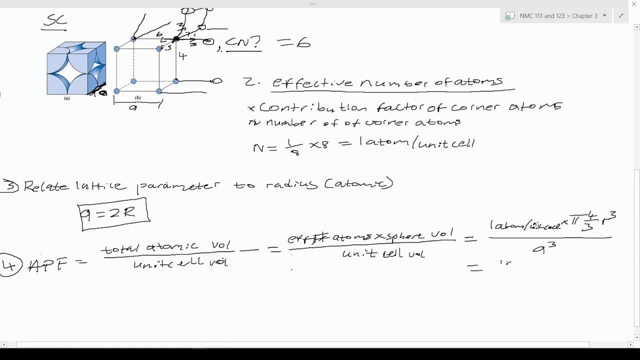 radius. so we have 1 multiplied by 4 over 3 PI R squared cubed, sorry. and then you have 2 R cubed and then the radius is going to cancel each other. so you'll have to 4 over 3, PI over 8. 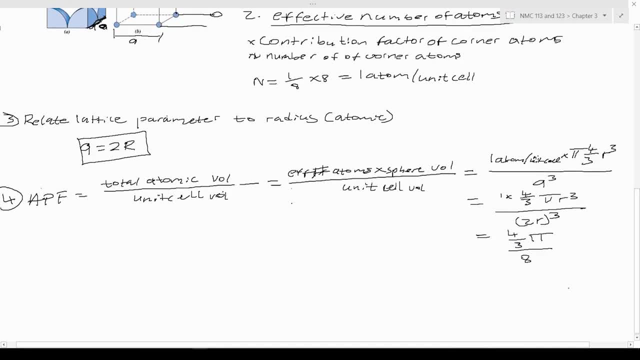 well, we go down a little bit. I mean, that's the atomic packing factor. if you resolve the equation, it's just gonna give you. you gonna, okay, multiply 1 over 8 with 4 over 3 PI. that will make it 1 over 6 PI. 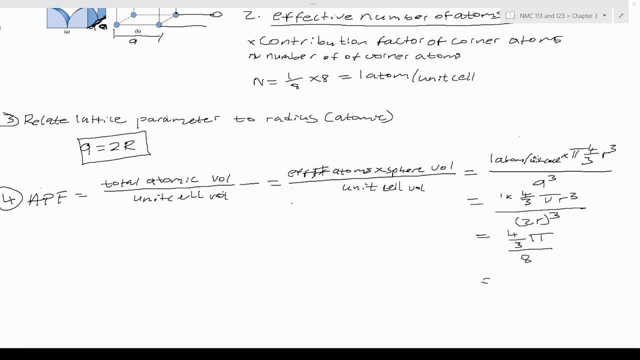 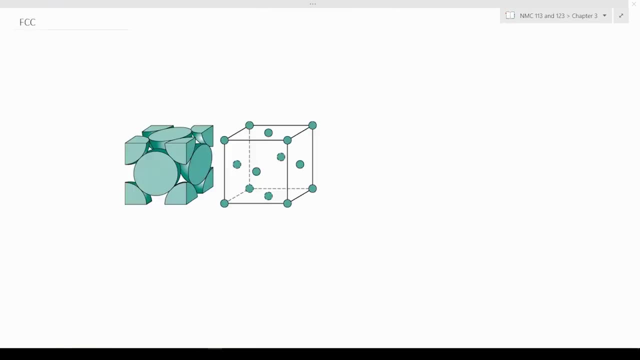 that would be your atomic packing factor for a simple cubic. ok, There you go. now let's actually take a look at the face-centered cube current. Now let's take a look at the face-centered cubic. For this particular one, you have body-centered- I mean face-centered- atoms on the six phases. 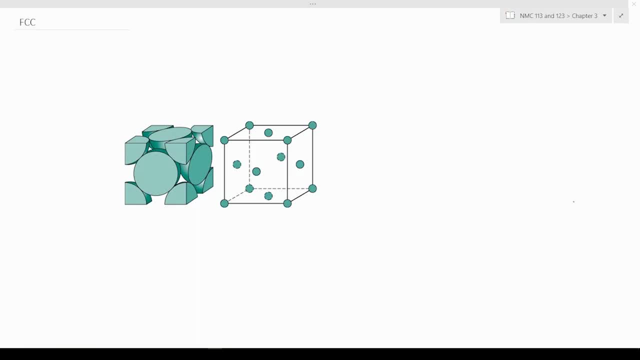 of a structure. So we're also going to determine what we actually worked out. for the simple cubic, which was the coordination number, I said that we choose a reference atom. In this case it's much easier choosing the face-centered atoms as your reference atom. 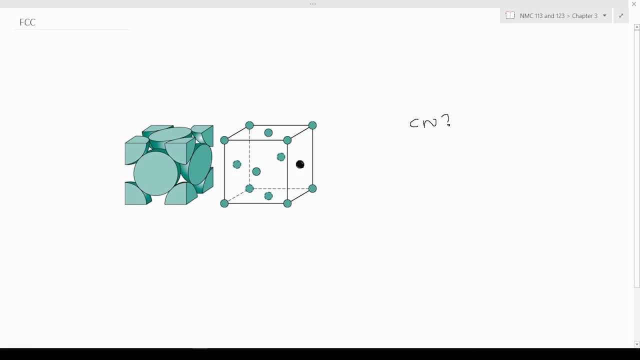 because they have. you know when you're making the count. it's actually much easier to make the count when you're choosing the face-centered atom. If you choose a corner atom, you're just going to make it difficult for yourself because and some of these atoms you may not find that it has as many nearest touching atoms. 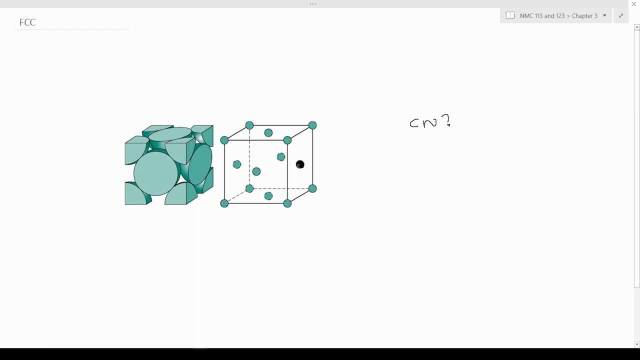 as the face-centered. So for an FCC, choose a reference atom of the face-centered atom. Now, if you extend these crystal structures to the face-centered atom, you're going to see that there's one that has formed into the right-hand side, the neighboring. 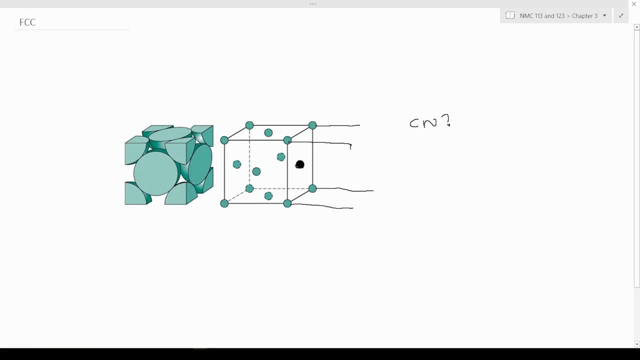 Let me just do this. Okay, you have one here, the front, one at the top, one at the bottom, one at the top, one at the bottom, And then you have one here. you have one at the bottom and then you have one at the. 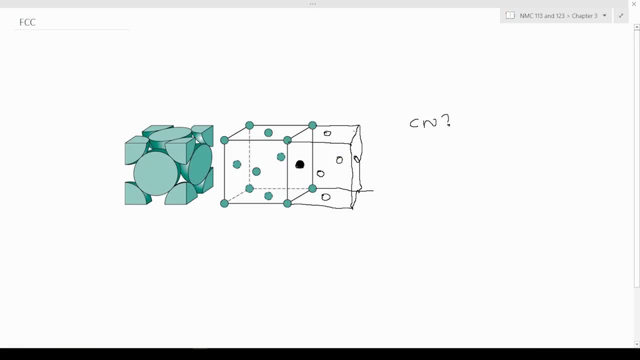 back, And then you have these corner atoms as well. Okay, when you're counting the nearest touching atoms, you're going to have to make sure that you have the right-hand side, Okay, And then you've gotta make sure that the next one, the one at the back, that's touching. 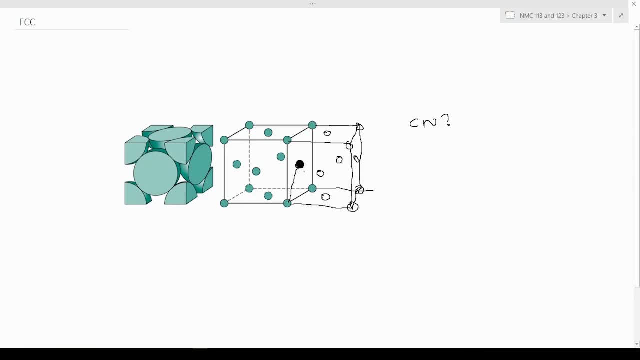 this one, right, This one. so it's one, two, three, four- my lines are not that straight, but as long as you can see, Okay, And then it touches the one in the neighboring side. Okay, neighboring cell, it's going to be five, this one, right, and then it's going to be six and the one. 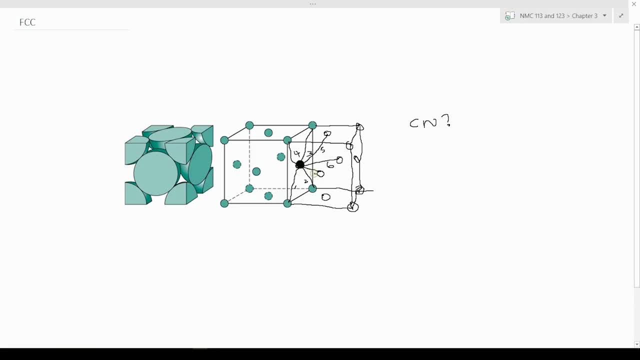 front, this is going to be seven. just write seven here. and then the one at the bottom, which is going to be eight. pay attention, like if you look at this, this, this entire structure, you'll actually see that because of these atoms that are actually touching it, this or the ones on these phases, the one86 at the face, at the back, this one, you do, it's not. 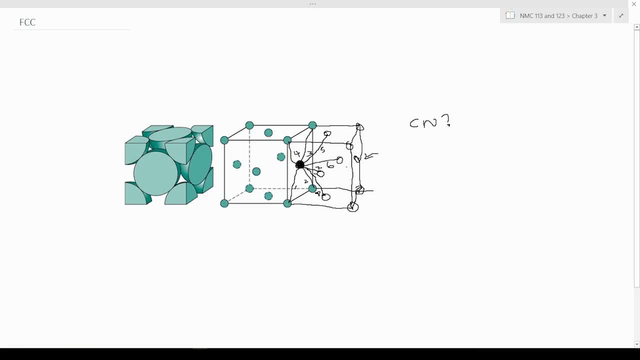 going to touch that happiness s, and we just chose. you don't be able to touch it, therefore not counting it, so now just have eight, and then going to the others, to the, to the, to the, our primary cell, the cell that wasn't really extended you have from here to here, so it's nine. 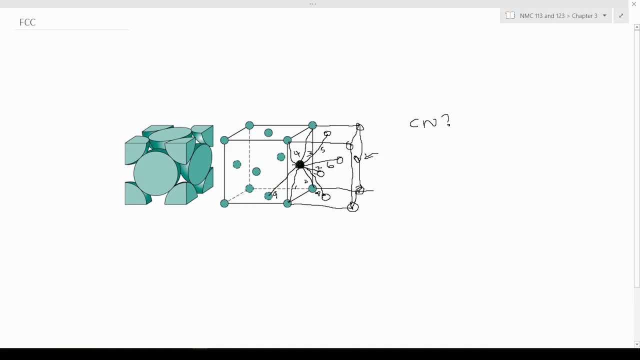 right to the one at the back, 10, the one at the top, it's 11, red, and then you have one in front. it makes it tough. so the coordination number for an FCC right, when FCC it has a coordination of all 12. I should hope that you understand this. most people just cram in the 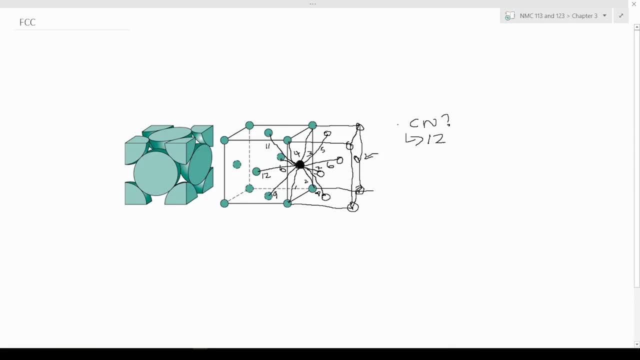 coordination numbers because you really just have- well you know- a limited number of crystal structures. but it's better to know how to make these calculations so that if they give you a structure you've never seen before- which doesn't happen that often- but you'll actually be able to make the 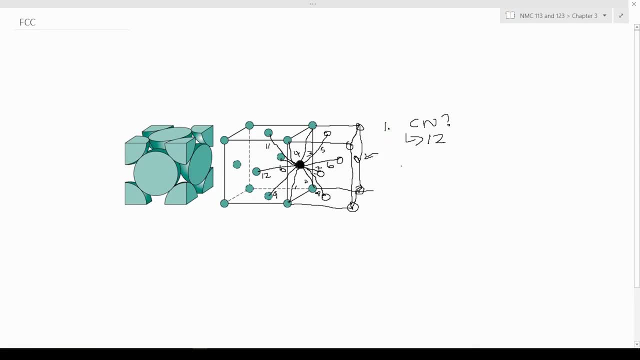 count to yourself. and then the second thing here is being able to count the effective number of atoms. okay for an FCC, being able to count the effective number of atoms. you have eight, eight corner atoms and then, uh, like i said, the first thing you do is to actually get the 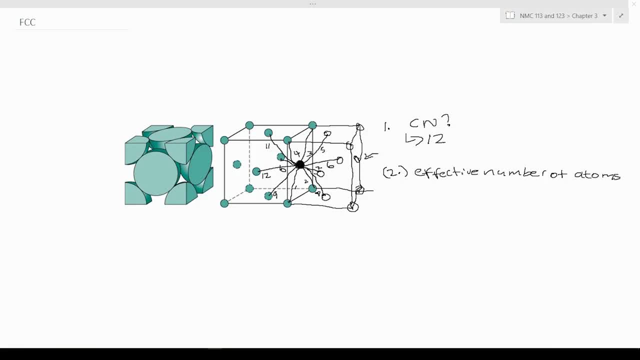 the contribution factor: right, my curse is eluding me terribly, so very terrible. okay. contribution factor of corner atoms: right, and then contribution factor, contribution factor, contribution factor, uh, the contribution factor. now we have face centered items as well of, uh, face centered items, face centered atoms. and then, after you do that, 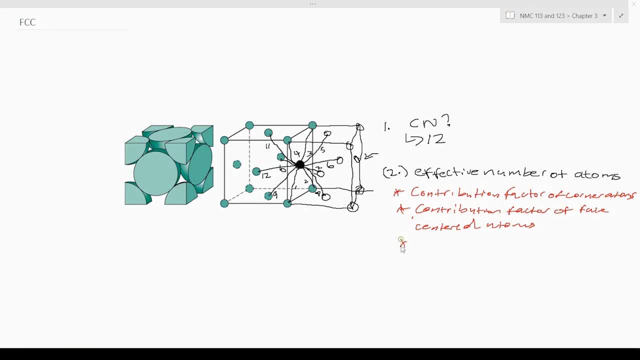 you actually get how many atoms, number of atoms- for each right, so how many contribution? i mean, how many, uh, corner atoms are there, and then how many face centered atoms are there. so this is how you get it. and then, uh, looking at this structure, uh, you'll just be able to see: 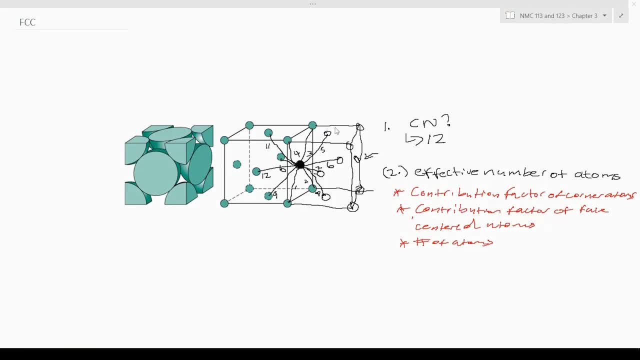 here you have um, six phases: this one, two, three, four, five and six right, so now you have uh, six, uh, face centered atoms, and then the contribution factor is a half because, like for example, this one is a half atom. you can see that it's, it's actually part of. 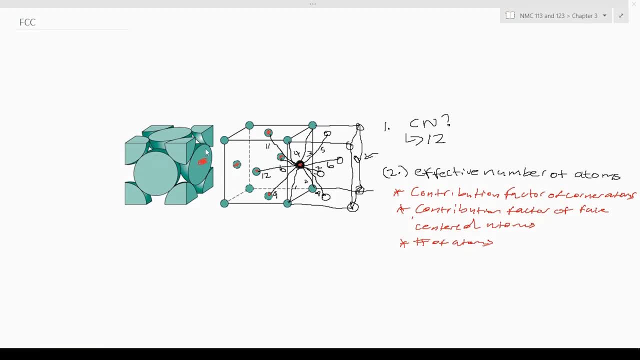 this unit cell, on this, on this it's part of this unit cell, соз cell, and it's only just half an atom. so the contribution factor of a face centered atom is a half. so you have for the face centered a half right contribution and there are six face centered atoms and in the corner atoms. 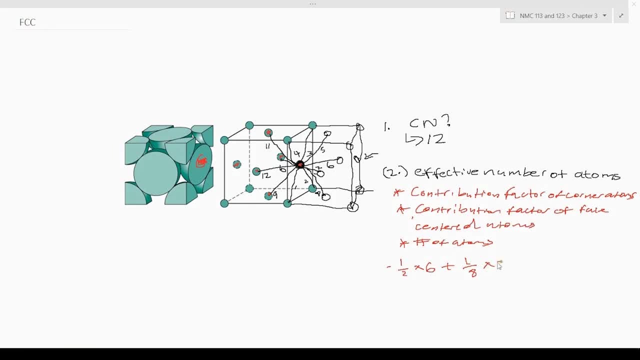 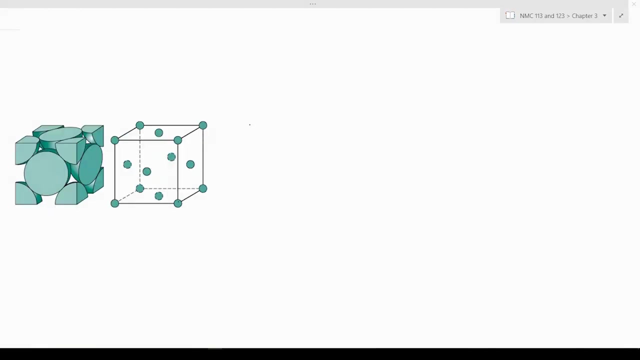 the contribution factor is an eighth and you have eight of them. so that makes that FCC has has two atoms, sorry it's four atoms, sorry it's four, because half of, yeah, half of six is three or four atoms per unit cell. okay, now the third thing we're going to be looking at. 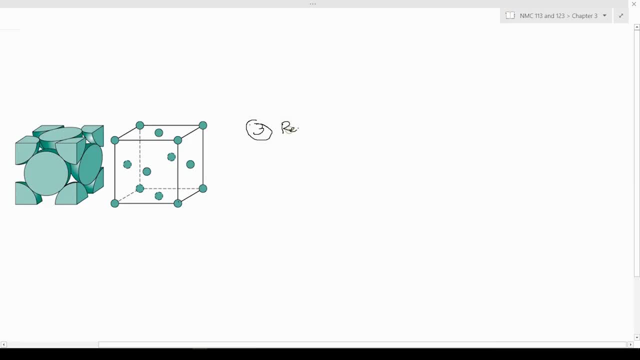 is relating the lattice parameter with atomic radius right. if you look to the drawing on the left or the picture to your left- the left most picture- you'll see that the fattened elements show up in this form. This here's the radius, this is two radii and this is another radius. and then you have 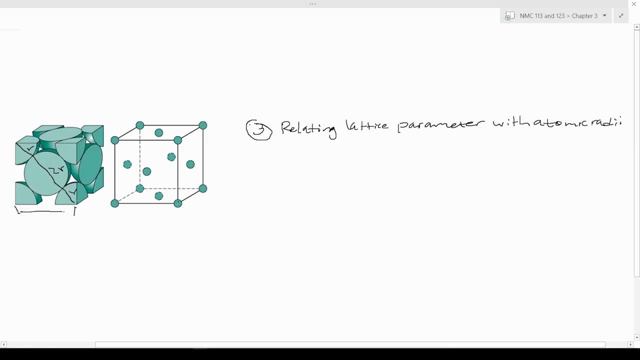 this A here as your lattice parameter. so, and then on this side as well, you have A. okay, you have A on this side. so for you to be able to relate these, just use Pythagoras theorem. Here's Pythagoras theorem. it's going to be four: R squared equals to A squared plus. 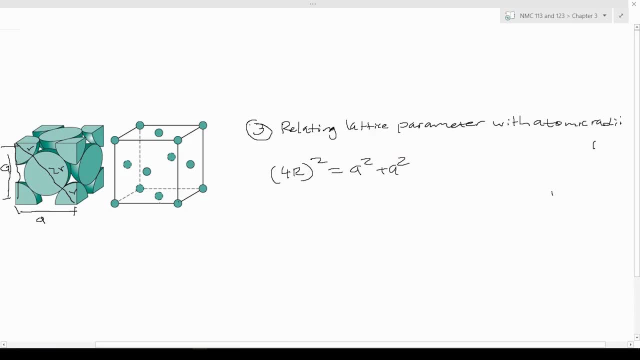 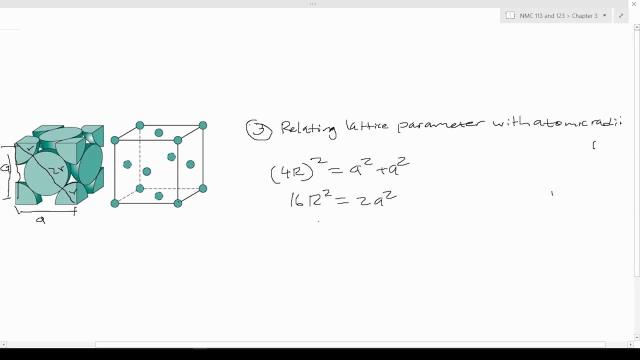 A squared, and then you have, well, 8 R squared, which is equals to A squared. so if you find a square root on both sides, you'll get 2, so 2 R equals to A. so this is the relationship. 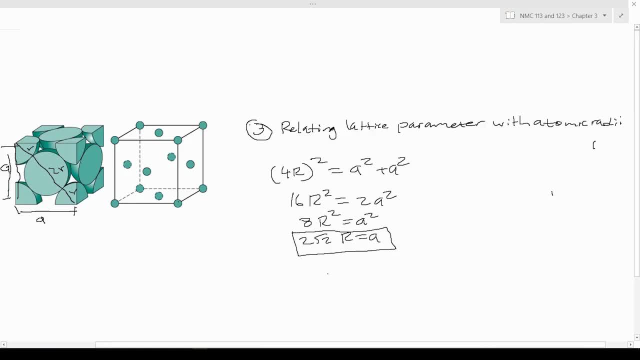 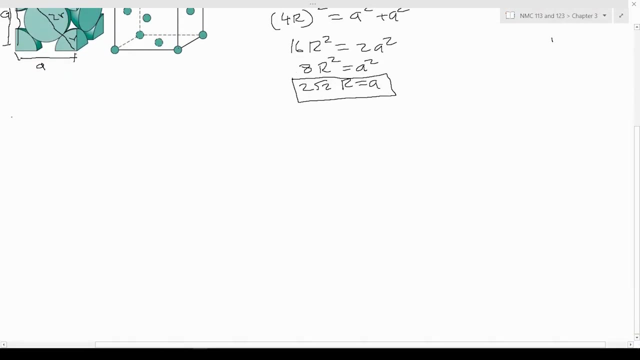 that the lattice parameter has with your radius, and you'll actually be able to use this relationship when you're calculating the atomic packing factor. so let's just do that. let's get the atomic packing factor. That's the fourth thing that you need to be able to do, right. 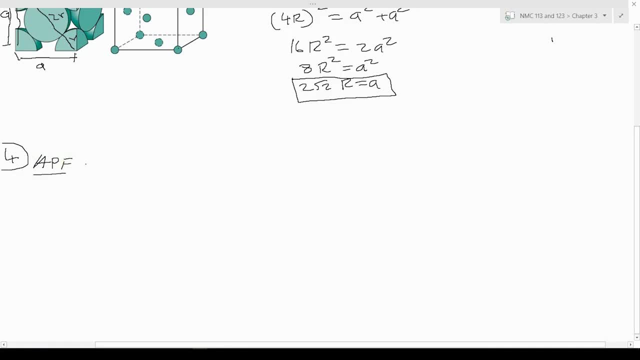 Atomic packing factor and we said that it's the total total atomic volume within the units and the cell volume. let's just say unit cell volume. okay, We just calculated the effective number of atoms. let me just rewrite the formula effective. 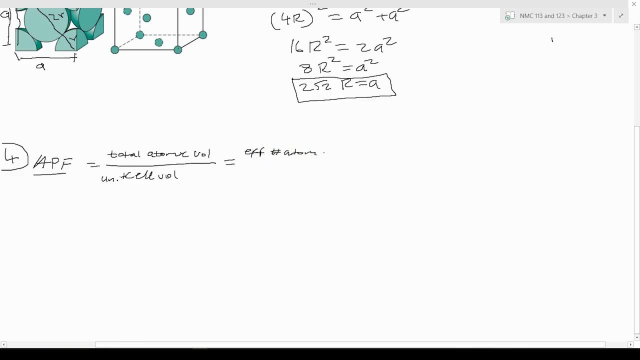 number of atoms times the volume of a sphere. Okay, Okay, Okay, Okay, Okay, Okay. And then again, unit cell volume. And what we have here is, for an FCC, we have 4 effective numbers of atoms, right. 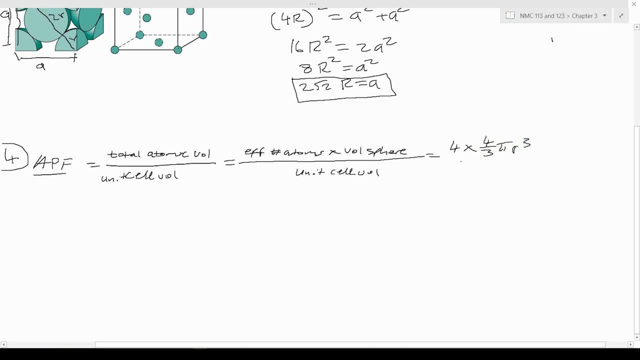 Atoms per per unit cell, And then 4 over 3 Pi, R cubed is the volume of a sphere. Then you have a sphere. the volume of a sphere after E squared, R cubed is the volume of a sphere. and then again an area of the mass of power equal to t, $2Weak clear left. 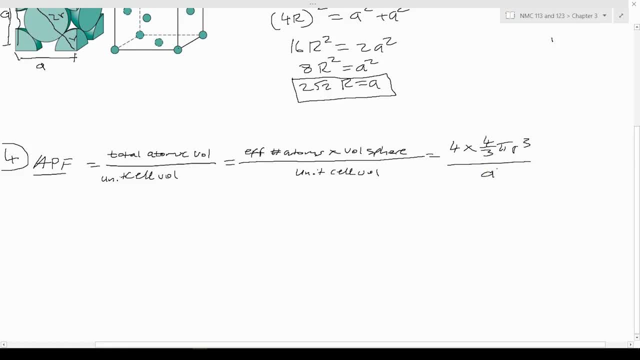 t Z square. we have a petal now ordered across here, so you can see that it's clear: High hand value. now ket a bar to continue. if it fails now, indeed, is a variable NP to then we have a cubed again because, uh, the shape of the unit cell is in term, in, in.